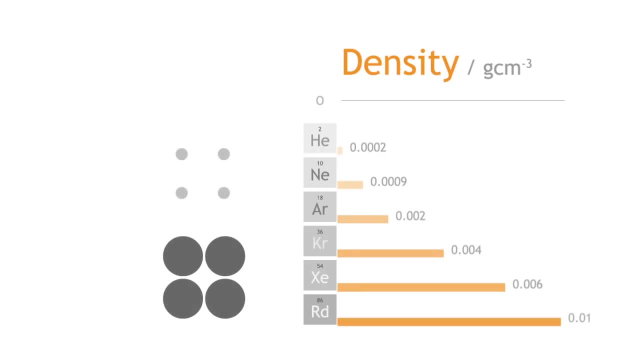 increases because larger atoms take up more space in a set volume, Since they are very stable and are hardly reactive. as well as their individual characteristics, they are called the noble gases. The noble gases have many practical real-life applications. One you might already know is 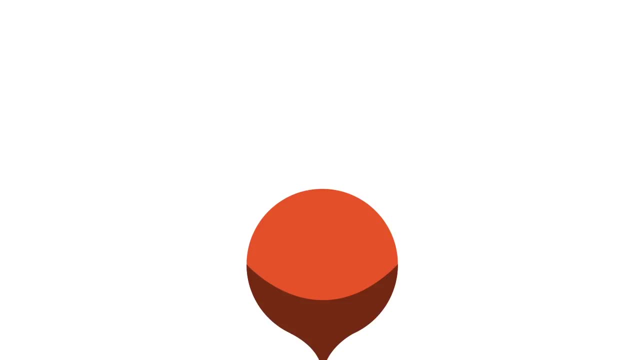 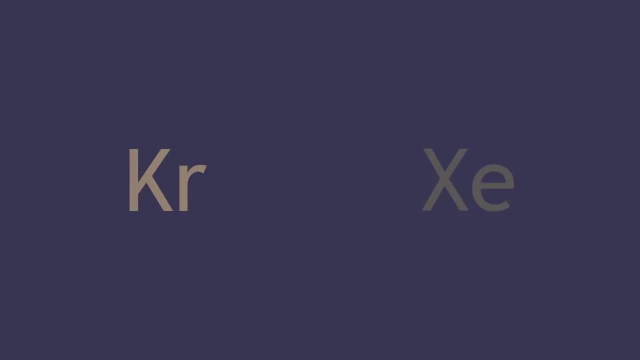 helium used to fill party balloons. Since it is less dense than air, these balloons float, And because of this property helium is also used to fill airships. There are actually many interesting uses in industry. Krypton and xenon are used in some types of lasers. 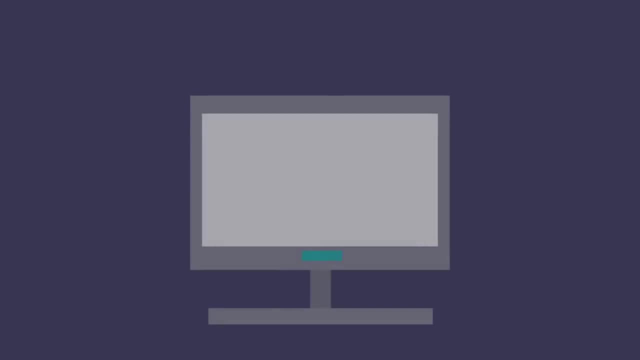 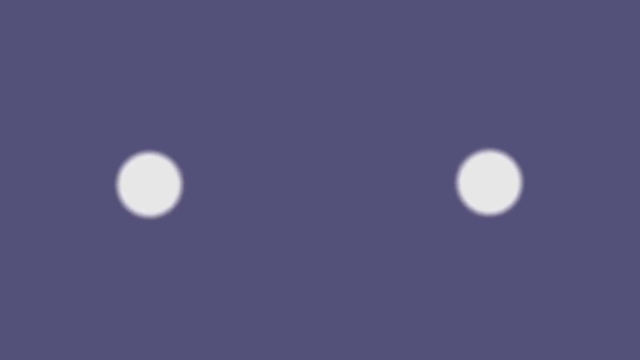 and in flat-panel display manufacturing. Since the 1990s, xenon is being used increasingly for car headlights to increase road safety. Xenon lamps produce a very bright light and increase contrasts and color vision. Although it is very inert, when an electrical current is passed through neon, it emits a bright 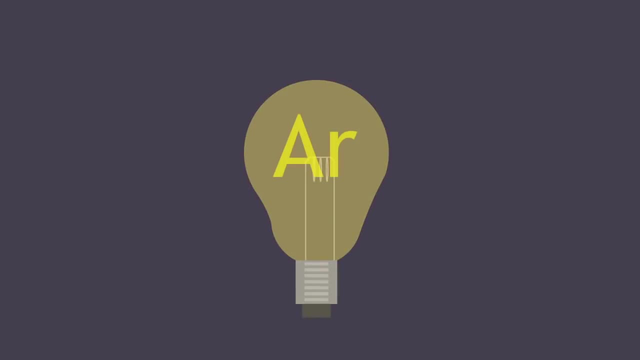 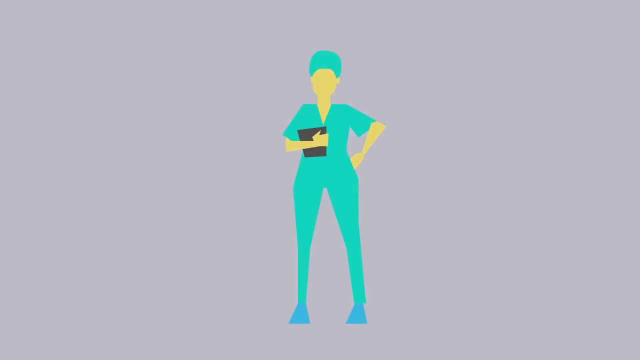 orange light Light bulbs are filled with argon. Unlike air, it will not react with a tungsten filament. Noble gases are also applied in medicine. Xenon is an effective natural anesthetic. It helps doctors maintain the patient's blood pressure and heart rate during operations and has particularly few side effects. Meanwhile, 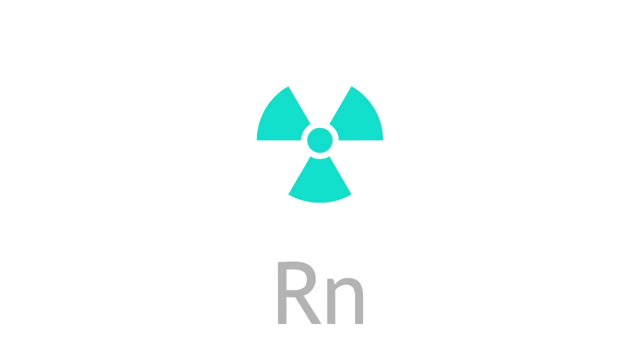 radon is highly radioactive, which is a characteristic that has been put to use in radiotherapy in attempts to cure cancer. These are the traditional uses of noble gases, But it even goes beyond that. Krypton is sometimes used as a filler in phytochemicals, an active force in human cells. These are the main uses. 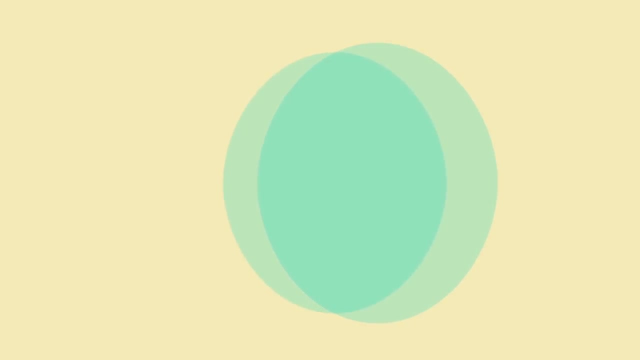 of noble gases. But it even goes beyond that. Krypton is sometimes used as a filler in the in double glazing set between two glass panels, krypton will offer very good insulation because it has a lower thermal conductivity than the molecules making up the air. 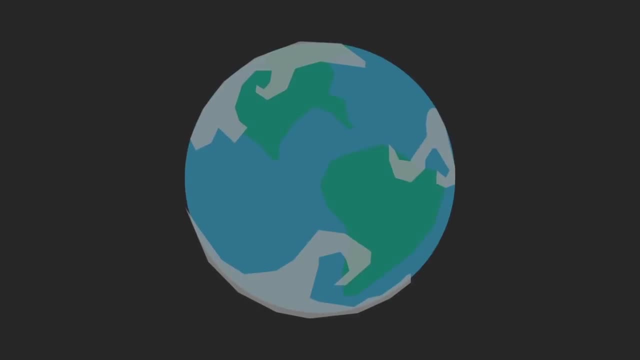 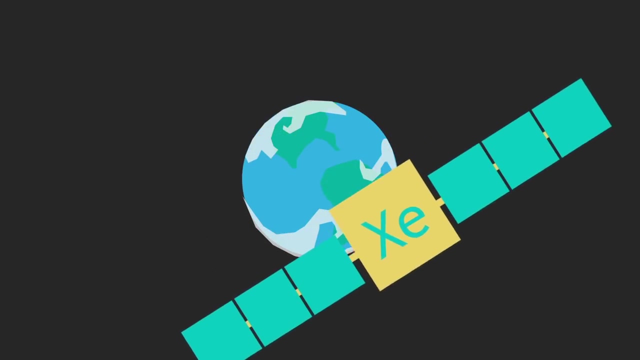 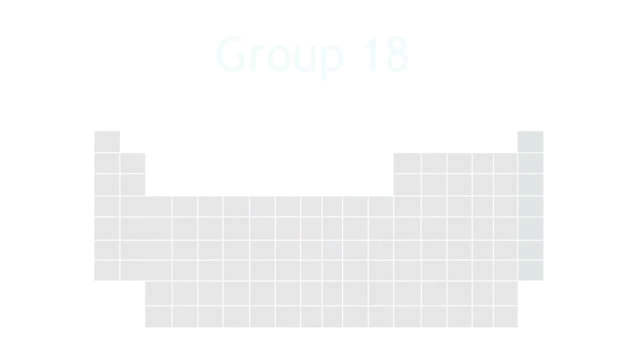 and it doesn't stop. in the space industry, xenon is used as a propellant that helps us steer satellites on their orbital paths. its mass ensures that we can put the satellite in movement. so now you know the basics of noble gases, the group eighteen elements, also known as group zero. their stability is one of their main characteristics, allowing for many real-life applications.